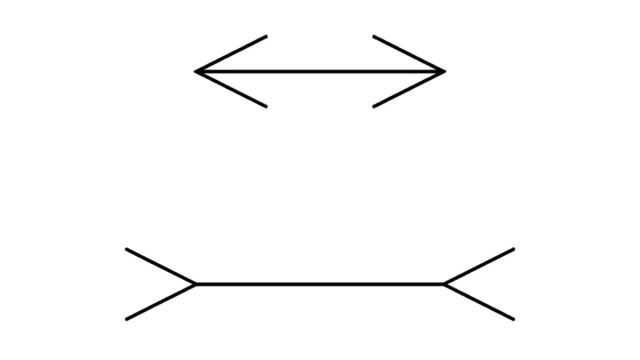 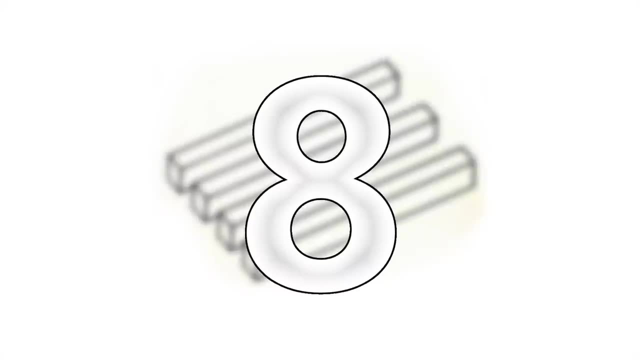 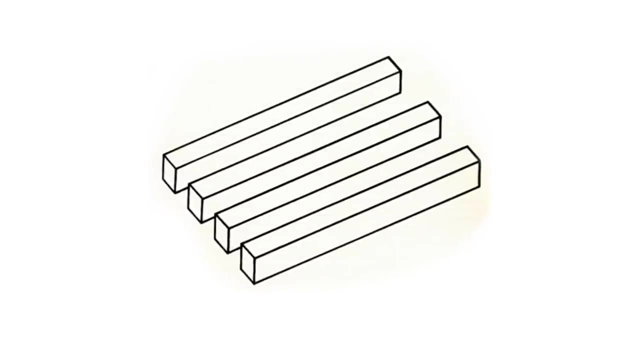 they are exactly the same. It's just the outside lines that make things complicated and create the visual illusion. Number 8 Coming in at the number 8 spot is a really old photo. however, till this day, it still confuses many people. Now, on one side of the photo, it appears that there are 3 planks of wood. however, on the 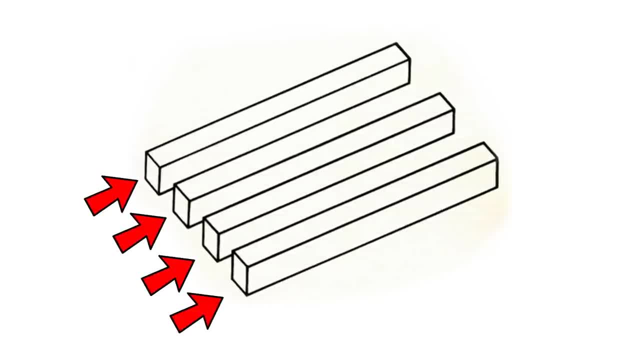 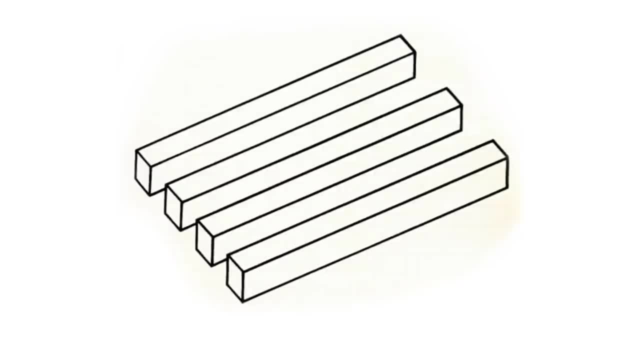 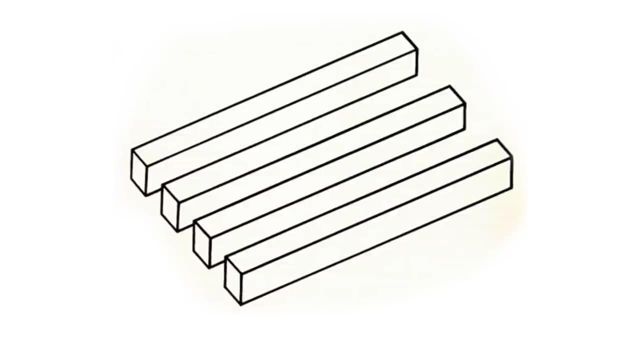 other side, it seems that there are 4.. So how many planks actually are there? Number 7, Now. if you're observant, you should have seen the extra line in the middle, and so, because of that, there are neither 4 or 3 planks. but 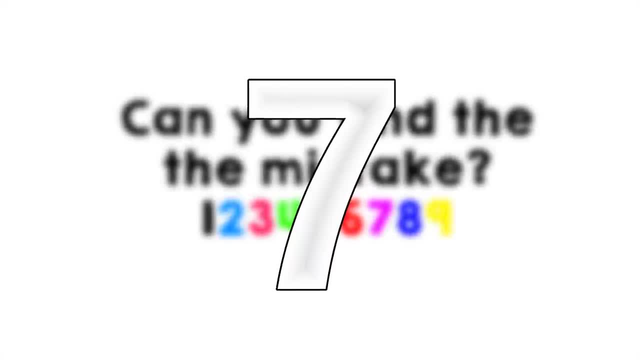 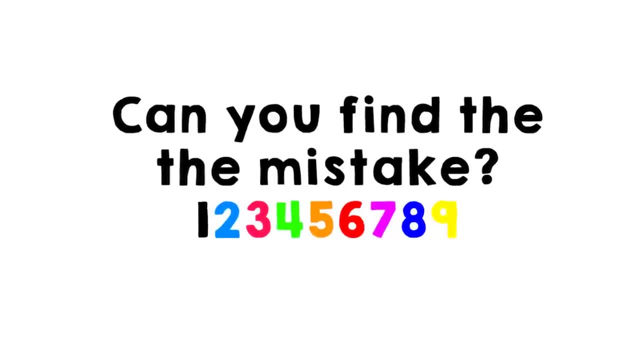 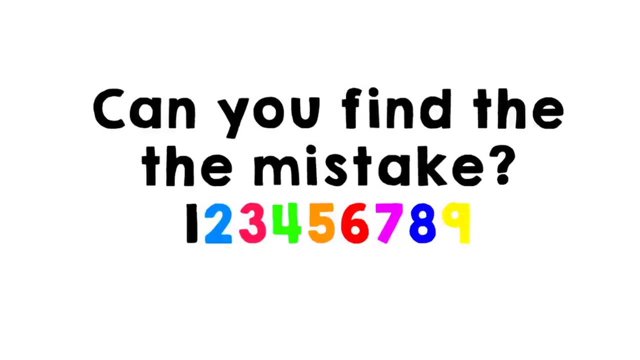 in fact, there's none at all. Number 7: Now for the number 7 spot. just try to spot the mistake hidden within this photo. Now, although everything seems to be fine, there is in fact a mistake, however, not in the numbers, as most people would look. 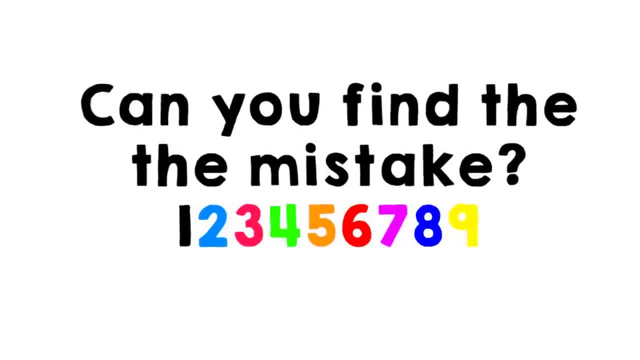 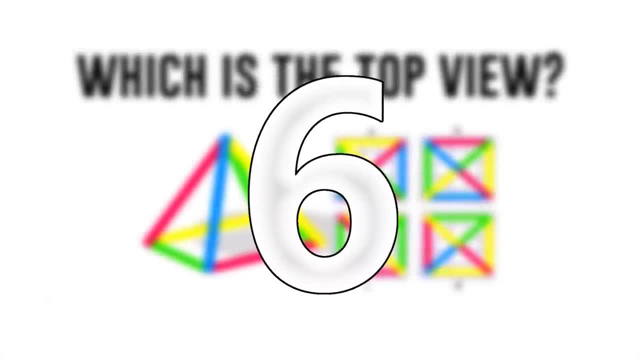 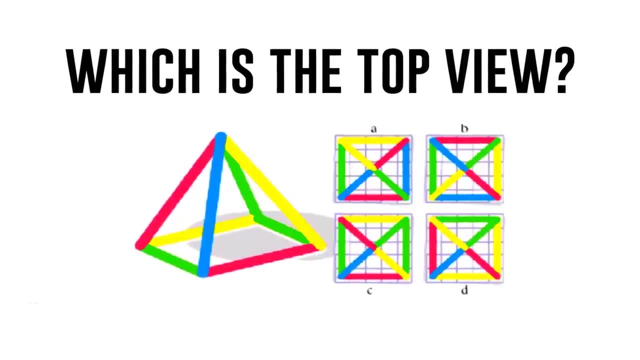 The mistake is actually in the question, as, if you look closely, there is the repetition of the word the right, after each other, Number 6. Now in this photo, you basically need to say which image is the top view of the diagram on the left. Is it A, B, C or D? 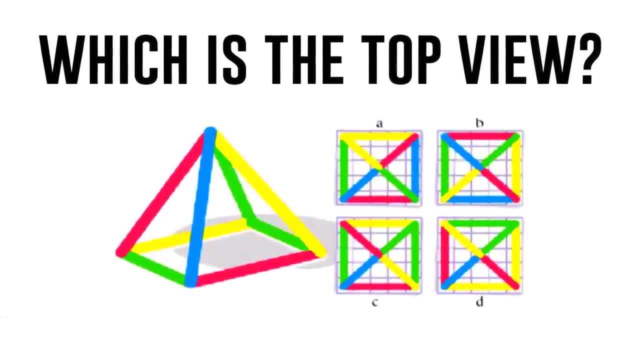 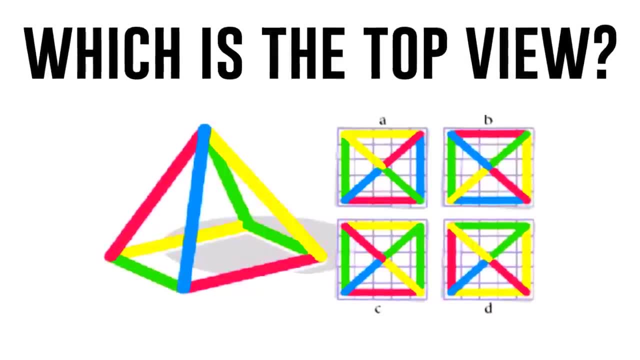 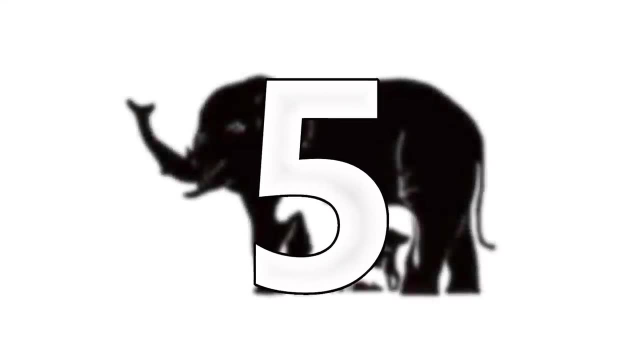 Number 8 Now, if you answer C, Then give yourself a pat on the back, as you are correct. The way to go around such questions is by basically visualizing the image and making sure all the colors match up. Number 5 Now in the photo displayed on screen, how many? 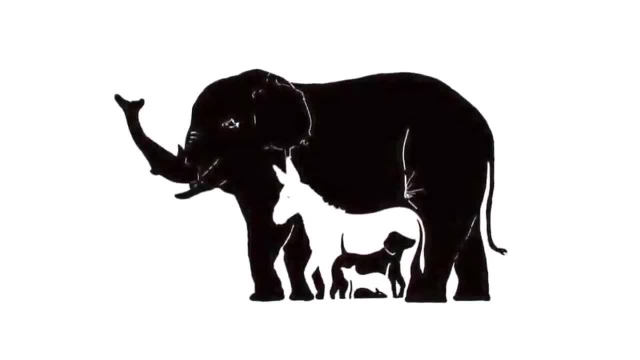 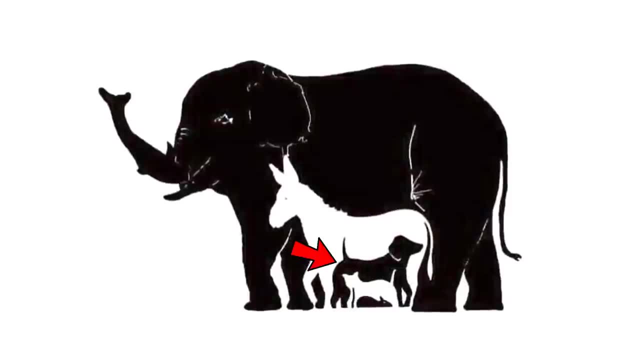 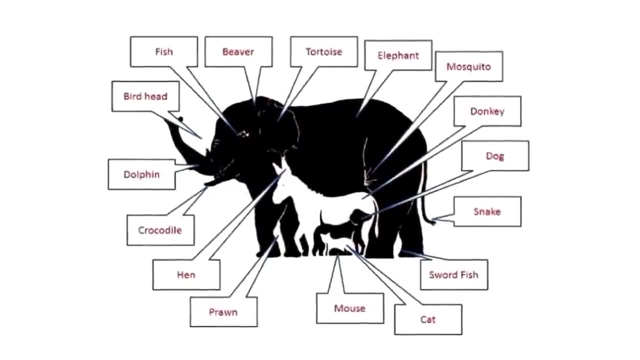 animals can you see? If you're like the majority of people, then you will most likely say 4, which are the elephant, donkey, dog and cat. How many animals can you see? However, in actual fact, there are 16 animals, as you can see pointed out on screen. 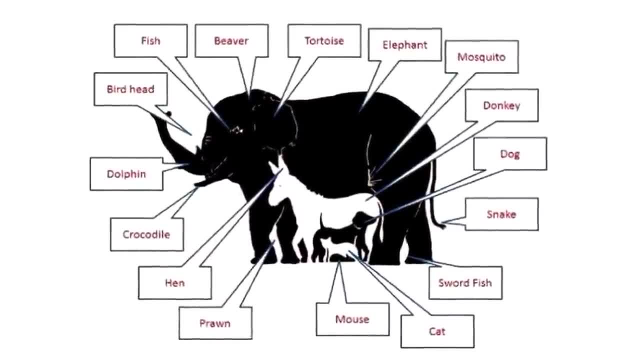 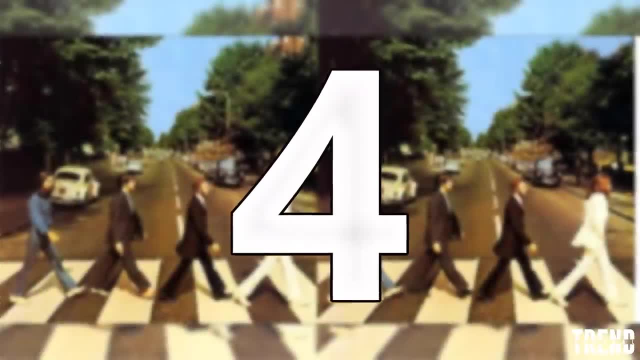 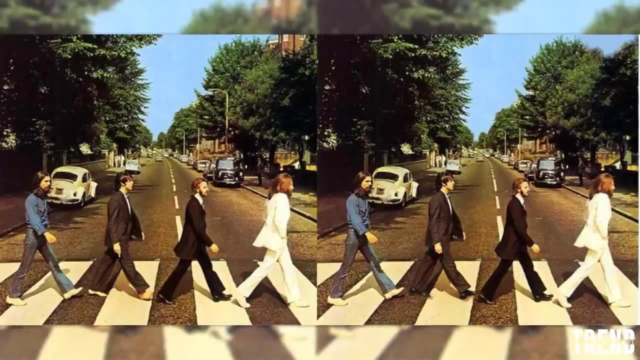 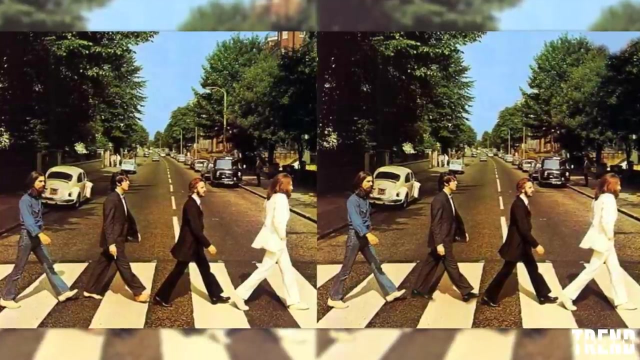 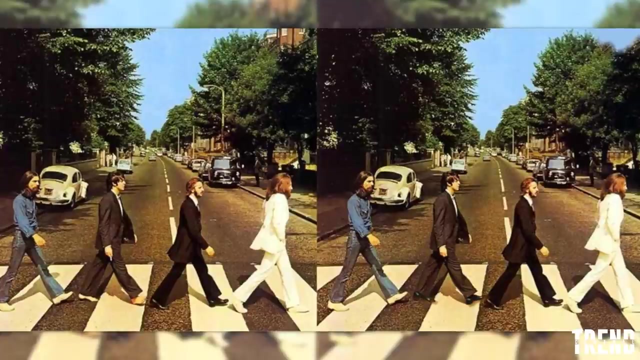 Did this one confuse you? Number 4 Now. the picture you see on screen now is basically an album cover of one of the best selling albums of the Beatles. Now, although the images are very similar, there are in fact some differences. Can you spot them all? 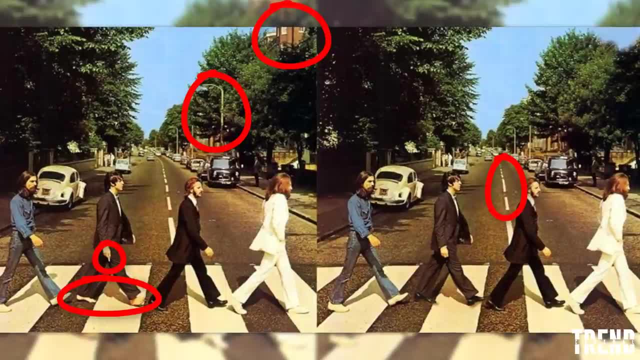 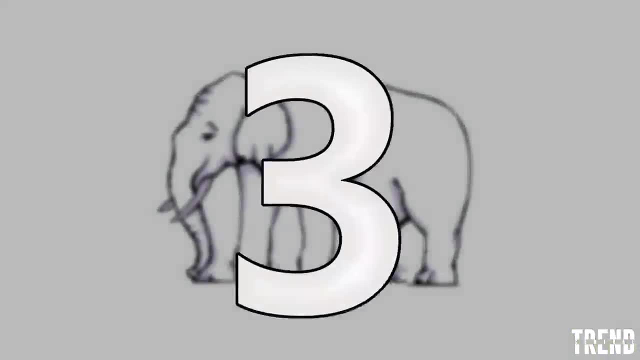 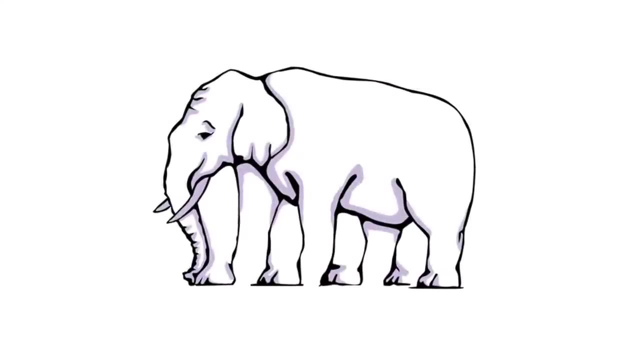 In total there are five differences, which are all marked just so you can compare with your answer. So if you did spot all the differences, then you truly are an intelligent person. Number 3 Now: in the photo you see on screen now, you should be seeing a picture of an elephant. 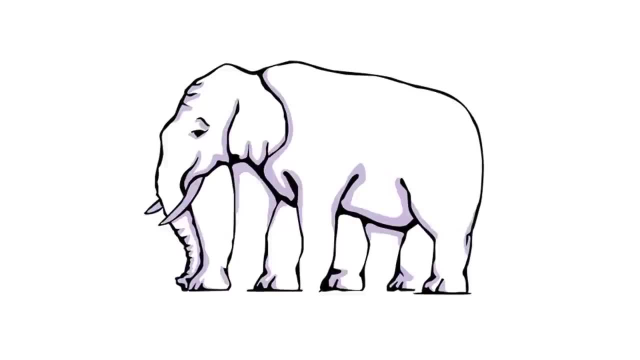 Number 3 Now in the photo you see on screen. now you should be seeing a picture of an elephant- Number 3 Now in the photo you see on screen. now you should be seeing a picture of an Elephant- Number 3 Now in the photo you see on screen. now you should see a picture of an elephant. 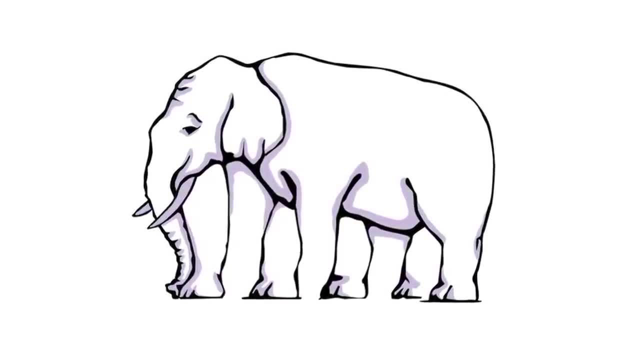 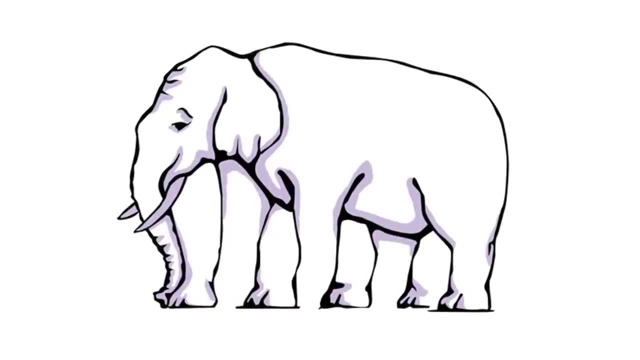 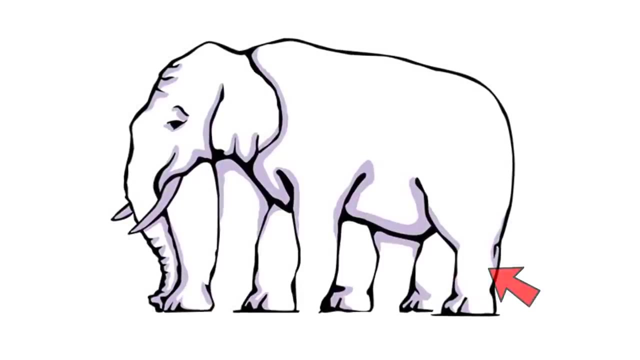 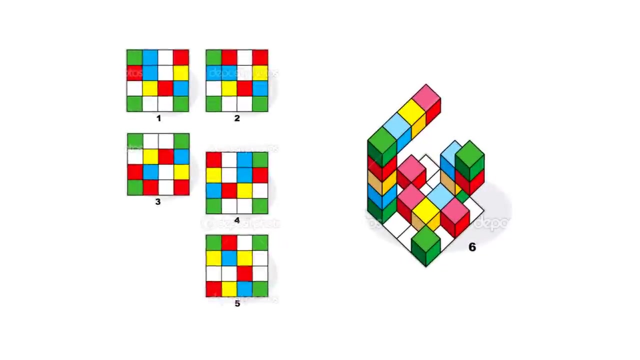 Number 3: You can also varyingly see a sự ヽ ノ. With this set of photos, you feel maybe the same, but much different. What do you guess? Number 3, Anyway, Number 3? mberost top view puzzle, however, this time using squares rather than triangles. now out of. 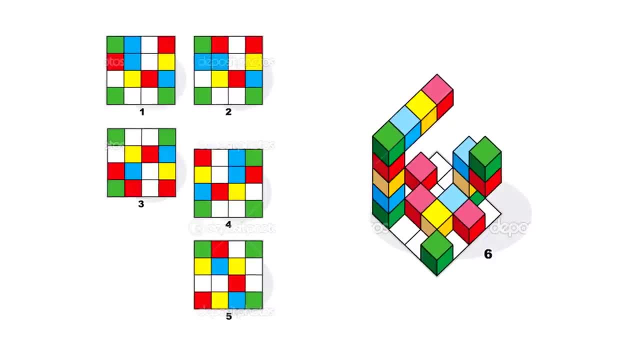 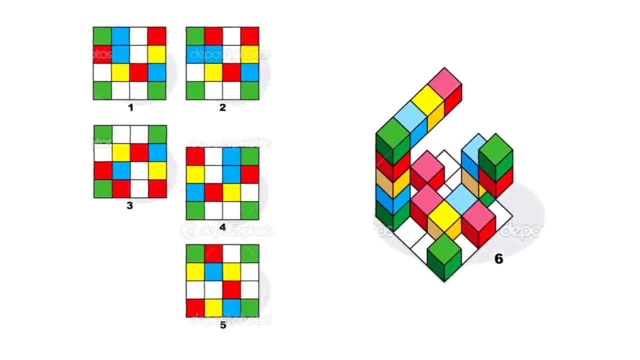 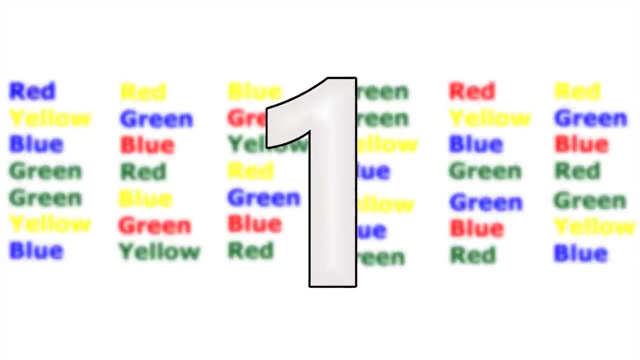 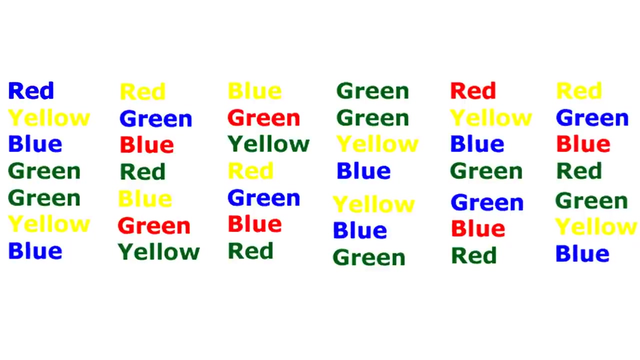 choices 1 to 5, which is the top view, to shape 6. if you guessed number 4, then you're correct, as it matches shape 6, exactly number 1. and now for the final photo. just look at the names of colors and try to say the names of the color. 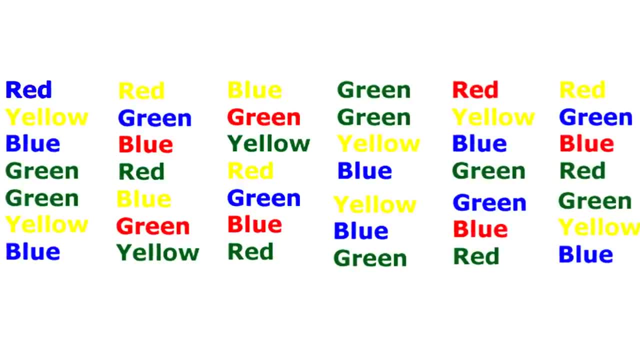 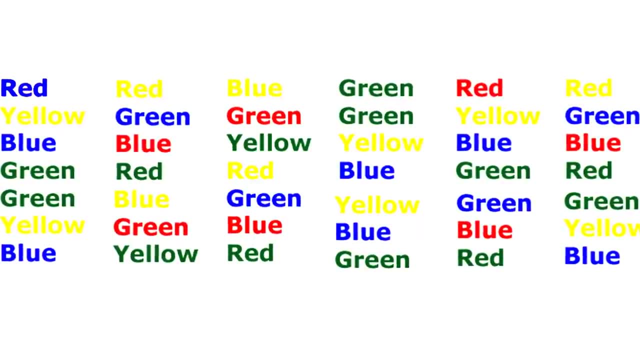 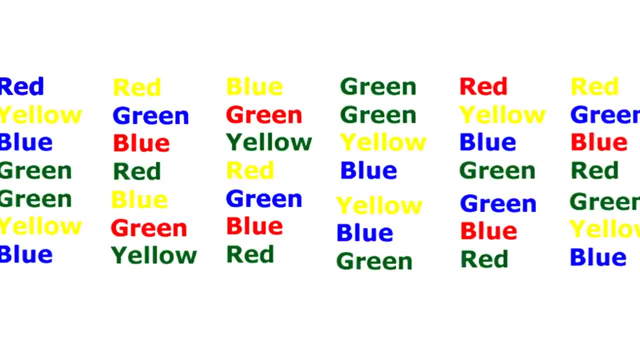 rather than the actual word. for example, the first one says red, however, you need to say blue. if you can complete the whole list in under 20 seconds, then you have a highly developed brain, as many people will fail to complete the list without making a single mistake.